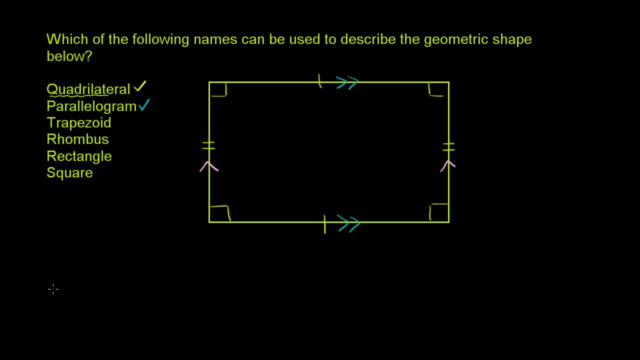 Sometimes it's defined as having only one pair of parallel sides. So let me write this down: Trapezoid, There's a debate here. It's not completely settled. Some people say at least one pair of parallel sides. That's one definition, one possible definition. 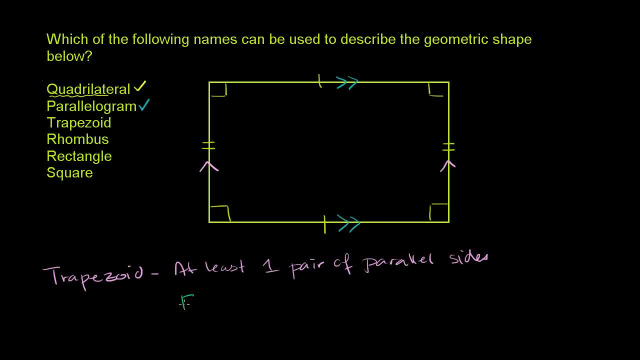 The other one is at exactly one pair of parallel sides, And this becomes which definition you pick. actually, How we answer this question depends on which definition for a trapezoid we pick. Now, the one that people most refer to is actually this one right over here. 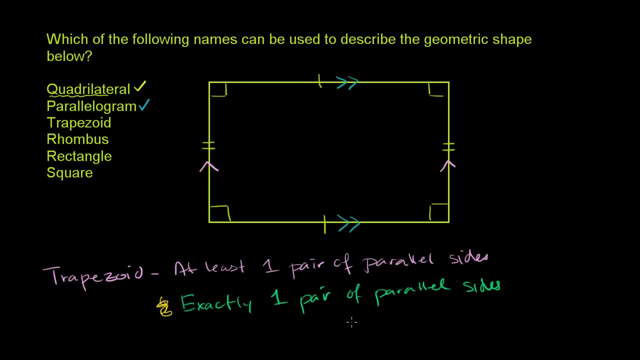 Exactly one pair of parallel sides. So the trapezoid that most people. when you think of a trapezoid, they think of something like this, where this side over here is parallel to that side over here And those two are not parallel. 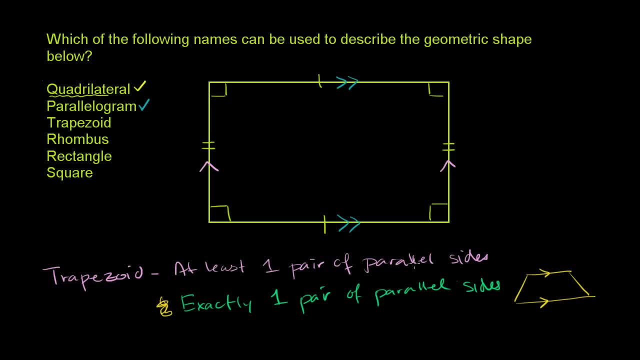 But sometimes you'll also see this- at least one pair of parallel sides, And so this would include parallelograms. It would be inclusive of parallelograms, because parallelograms have two pairs of parallel sides, But I'm going to go with this definition right over here. 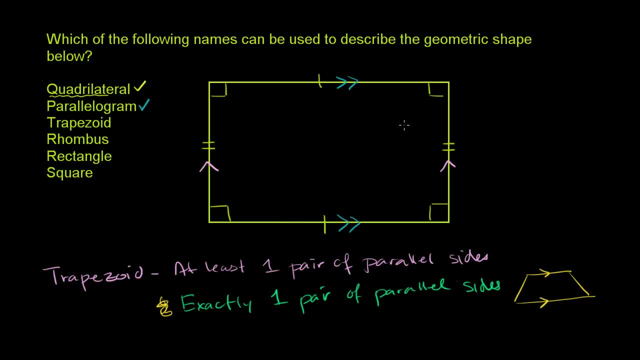 Exactly one pair of parallel sides. This has two pairs of parallel sides, So I will not call it a trapezoid, But it's always important to clarify what people are talking about, Because some people might say a trapezoid is. 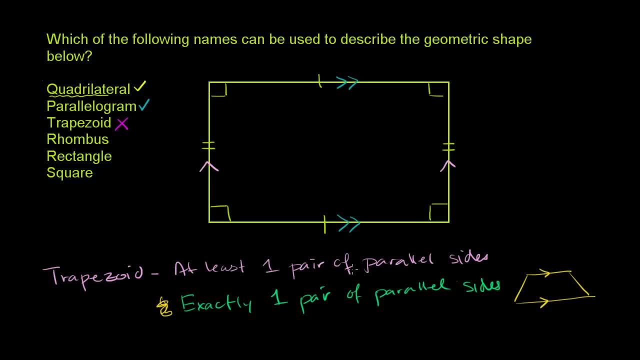 at least one pair of parallel sides, And if we used that definition, then we would call it a trapezoid. So it really depends on the definition that you're using. Now let's go on to rhombus. So a rhombus is a quadrilateral where four of the sides 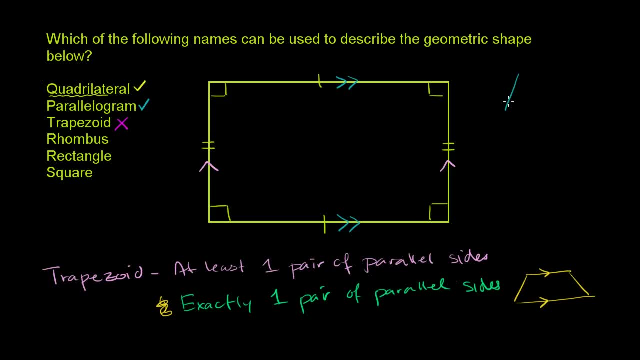 are congruent. So a rhombus will look like this: All four sides have the same length. They're not necessarily at right angles to each other. This figure over here. we have two pairs of sides that are the same length, But there's no information that tells us. 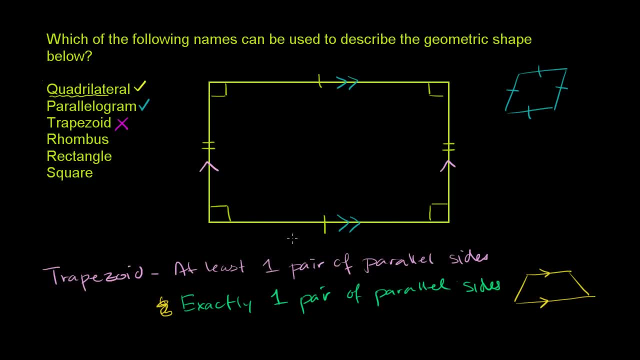 that this side is equal to that side or that this side is equal to that side. So we can't make the claim that this is necessarily a rhombus. We don't know for sure If someone told us that this length is equal to that length.